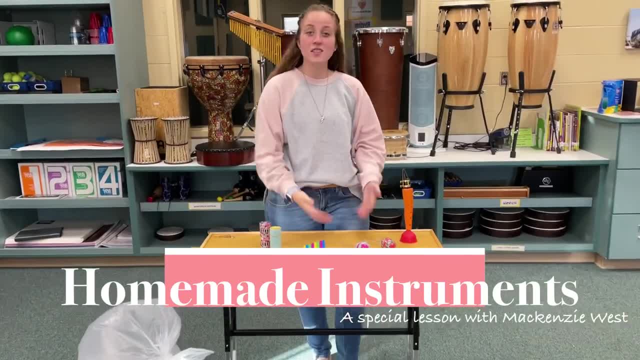 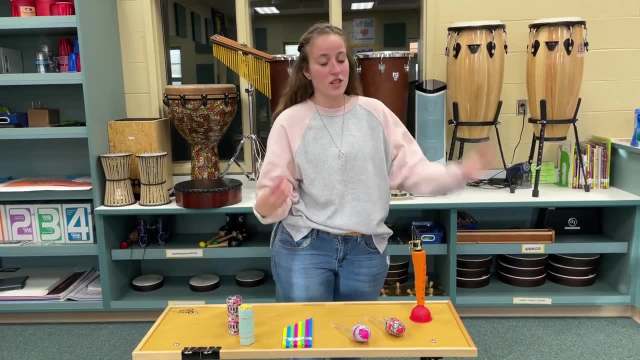 Hey friends, Miss West, here and today we're going to be talking about instruments that you can make at home. Now, believe it or not, you can make anything into an instrument, even some stuff that you have at home laying around the house. but I'm going to show you a couple examples of what you 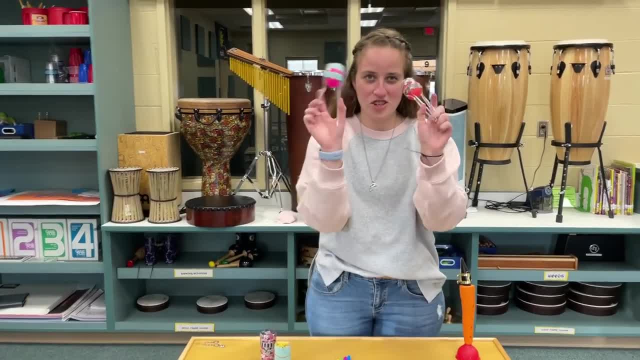 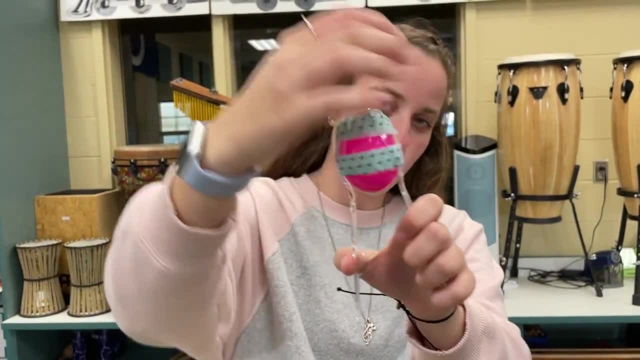 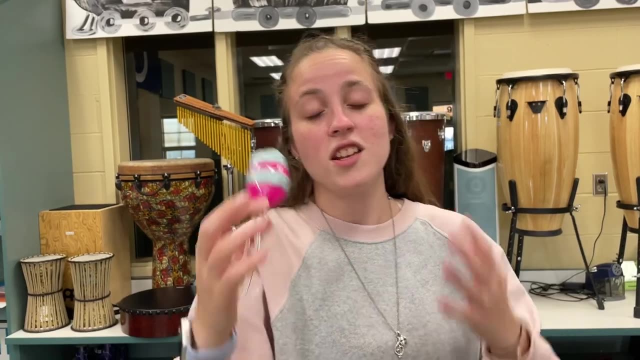 can do. So the first thing I have are some shaker eggs. Now, what I did is I took a plastic easter egg and I took two plastic spoons and I wrapped them around together with some tape, using washing tape. Now, the things that are inside the easter egg is some rice. Now, you could use rice. you. 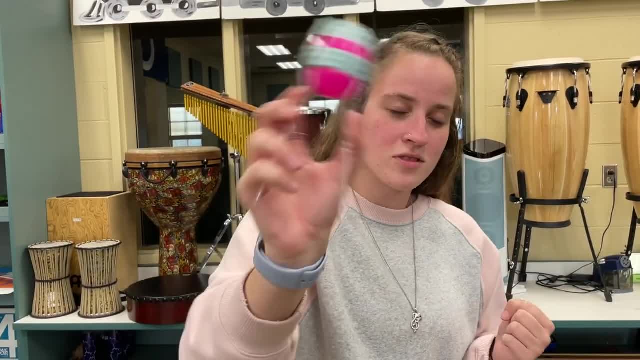 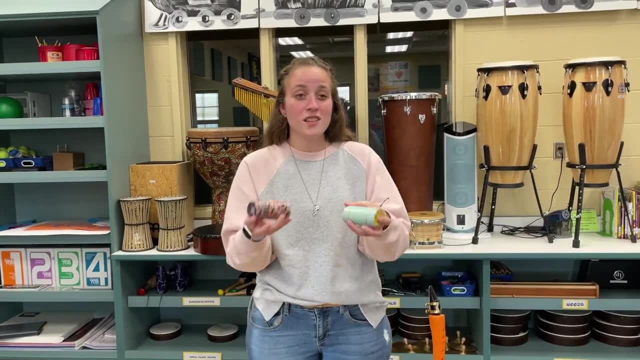 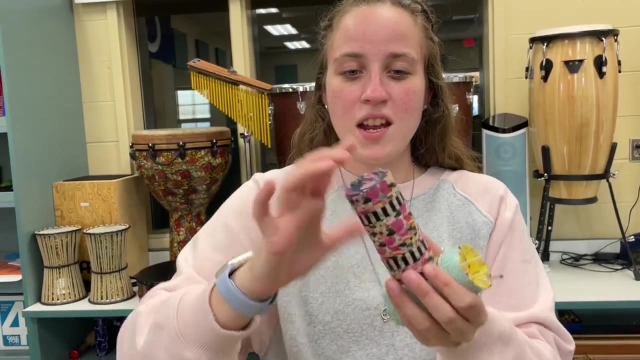 could use beans, you could use popcorn kernels, anything that sounds like a shaker egg- And the next thing that I did was I made some more shakers, but these are out of toilet paper rolls. Now I took two toilet paper rolls and I put some popcorn kernels in them and I taped each end. 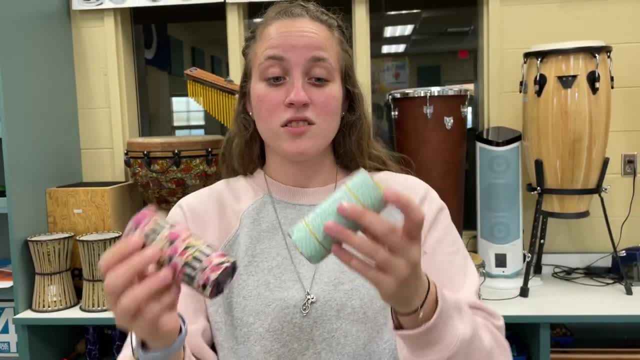 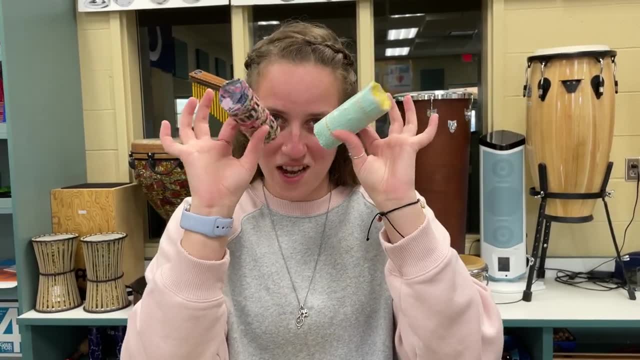 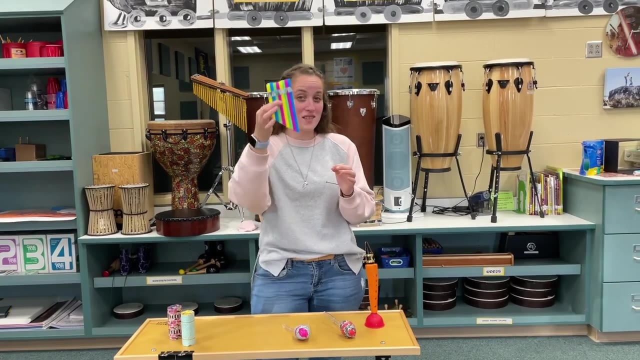 with some tape and then decorated it with washi tape So you could use markers, crayons, tape, paint- anything that you'd like to- to create and design your own toilet paper shakers. And the next thing that I did were some straws made into pipes, So I found some colorful straws. 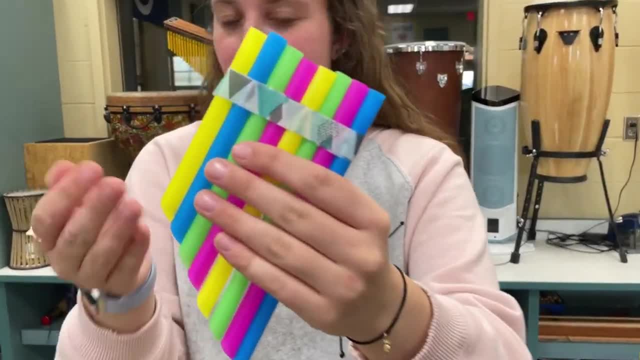 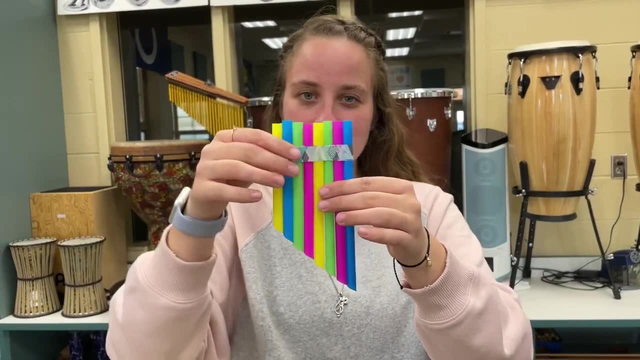 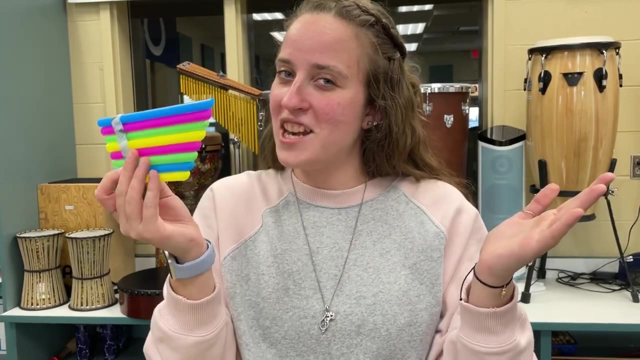 and I wrapped around with the washi tape again and I took some scissors- make sure you ask for help- and I did it at a diagonal so each of the straws sound like a different pitch. just like this. Pretty neat. You also can find some other other things around the house like this. I found a trash. 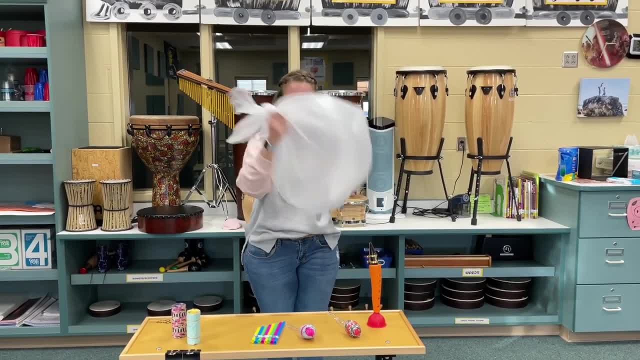 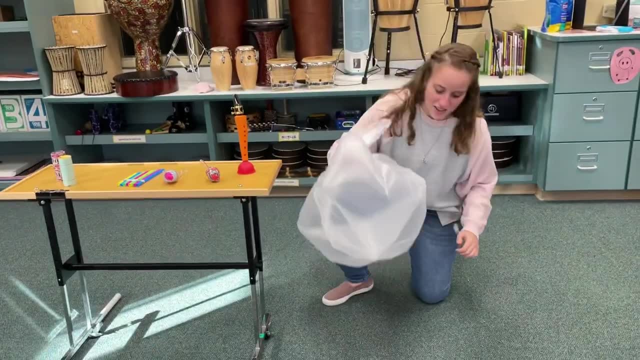 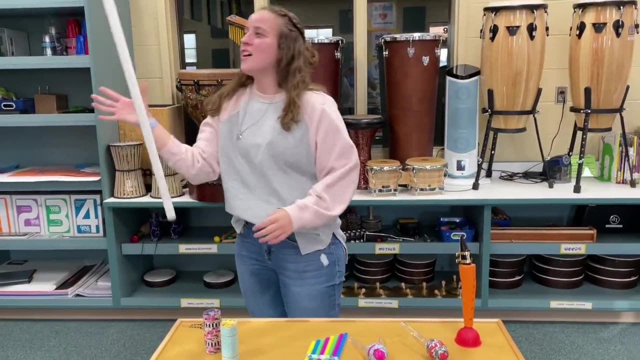 bag and I tied it off with some air in it and you can make it in into a drum, Even if I do it down on the ground like this. Pretty cool. Oh, I also found a PVC pipe. Now this I can make it into a drum. 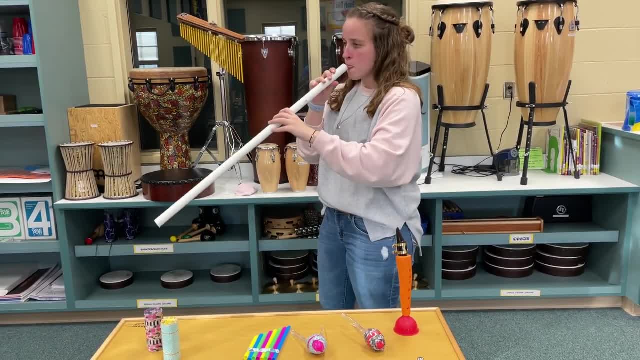 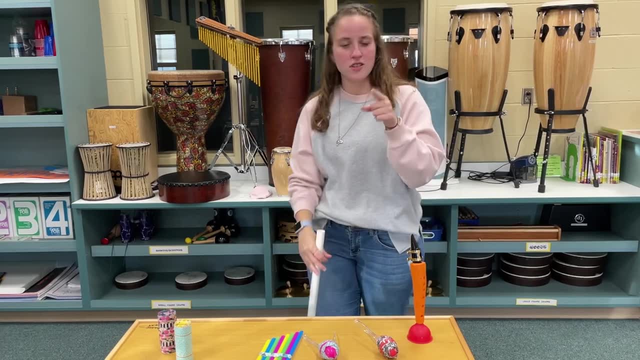 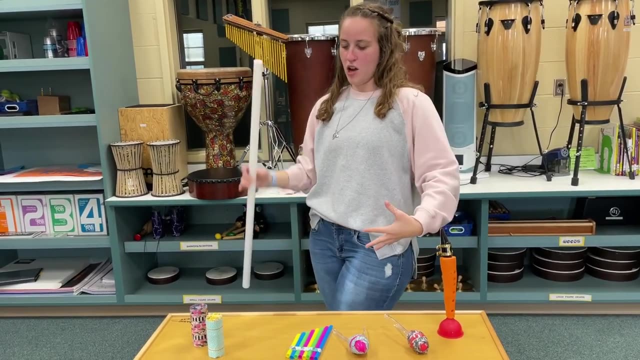 into a brass instrument If I do this, Pretty cool right? This kind of sounds like a didgeridoo, which is a really long piece of tubing, just like this in Australia. It makes such a low, deep sound Really fun. Last but not least, 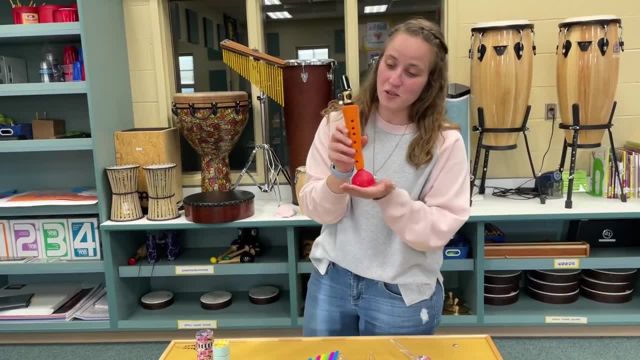 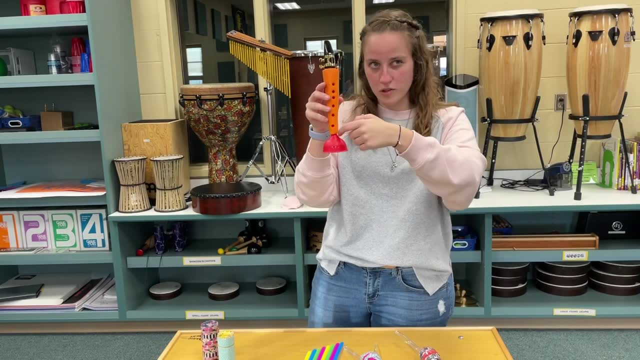 even you could use a carrot into an instrument, just like what Mr Doblesein did in his video about the carrot clarinet. So what you did is you took a carrot, drilled some holes into it, put a funnel at the end and got an alto sax mouthpiece. 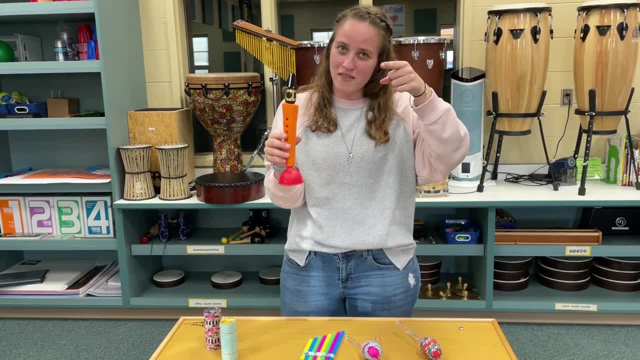 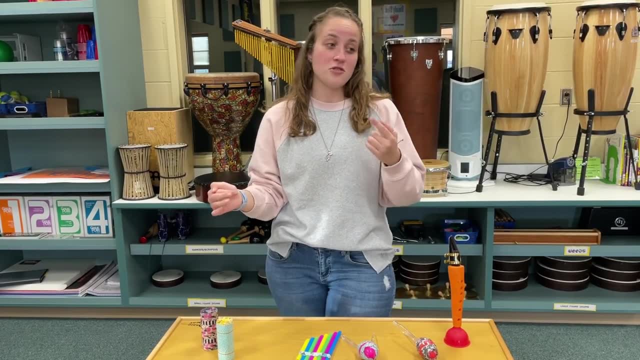 and it sounds like a clarinet. Make sure you check out that video. It's pretty cool, But anything is possible around your house to make it into an instrument. You could do some pots and pans, Anything that you want to do, But I want to see what you guys can come up with. Make sure you. 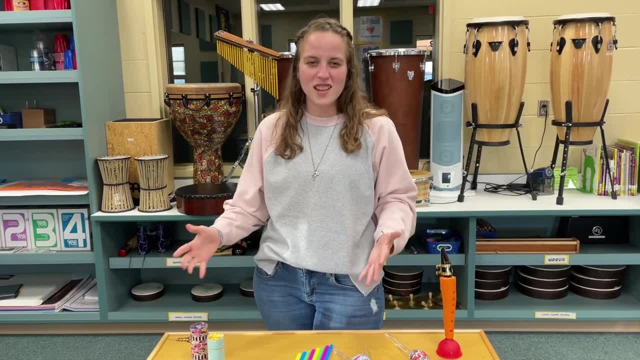 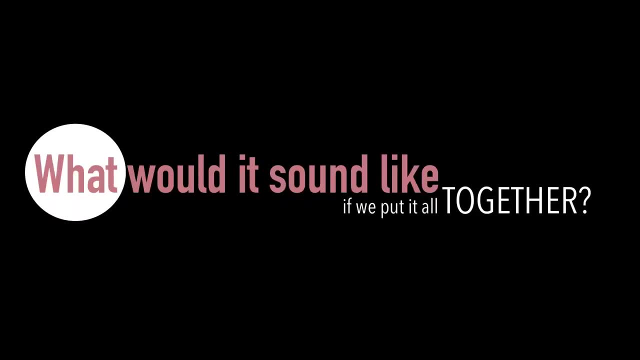 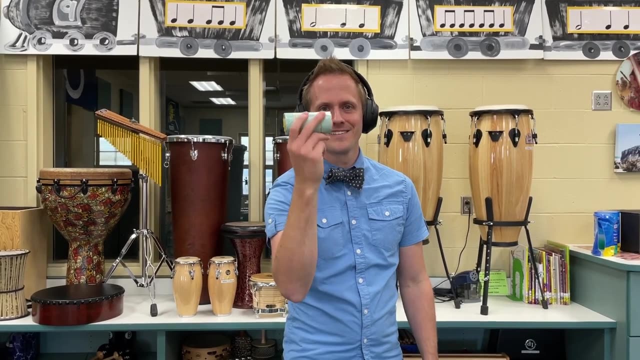 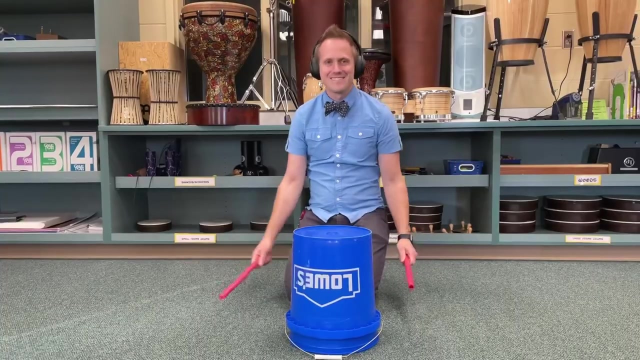 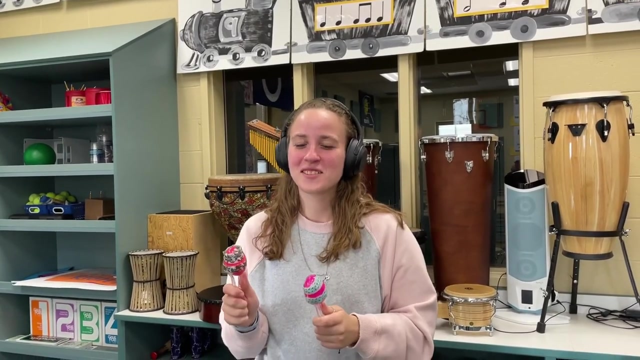 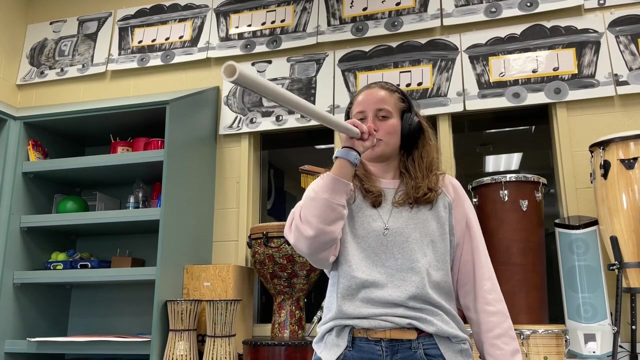 show me, Send me a video. Show, Mr Doblesein, anything like that I want to see. But for now, have fun creating and I'll see you guys later. Thank you so much for watching. I hope you enjoyed this video. If you did make sure to hit the like. 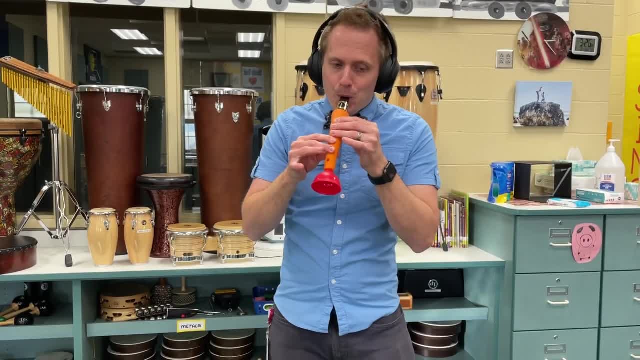 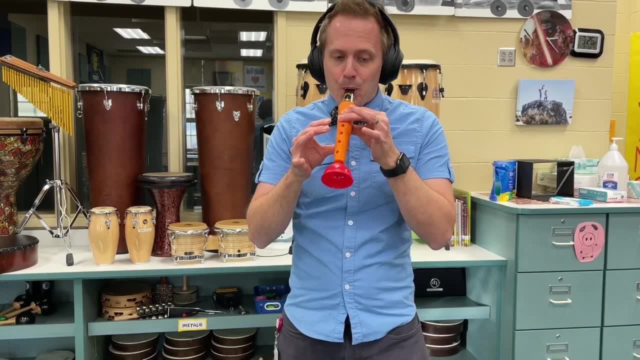 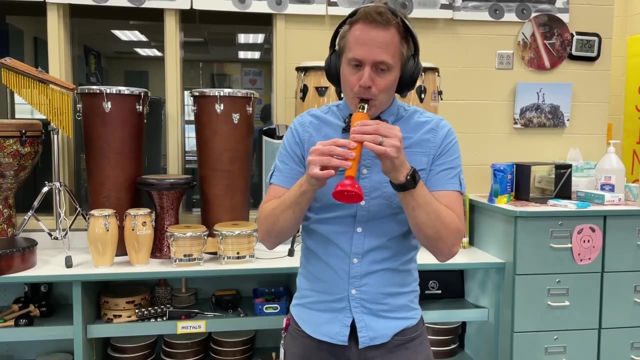 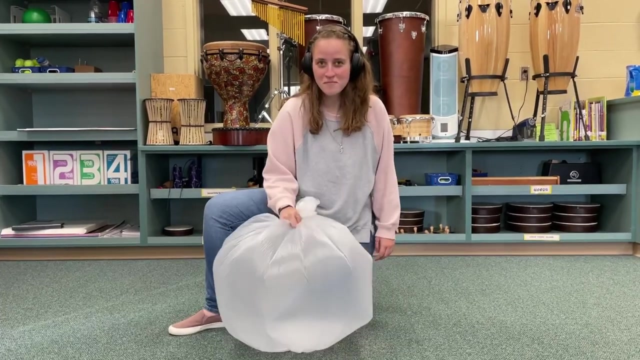 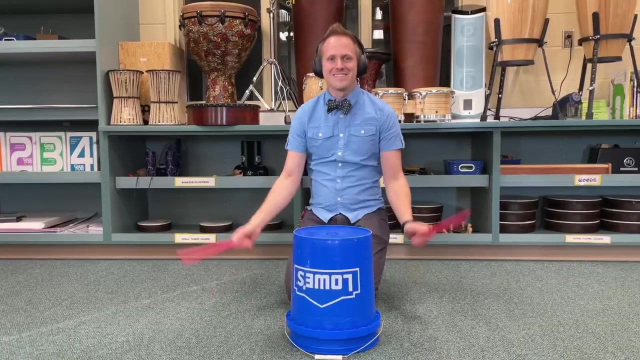 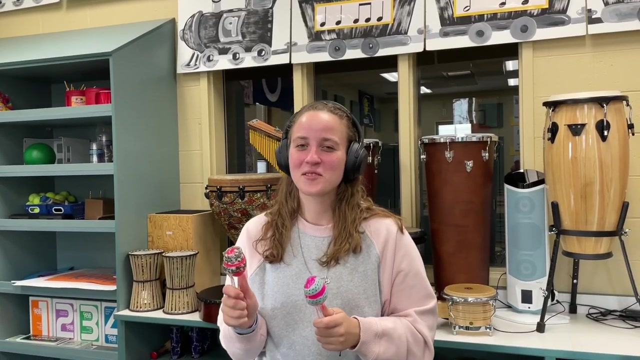 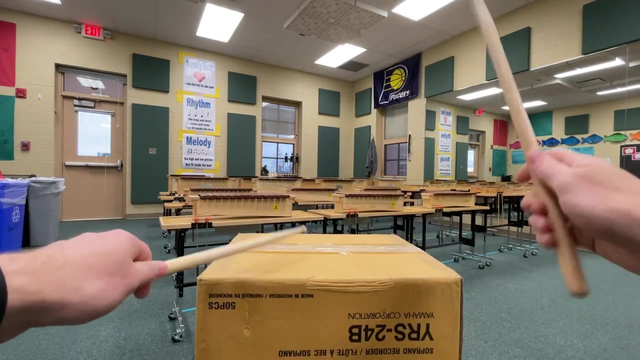 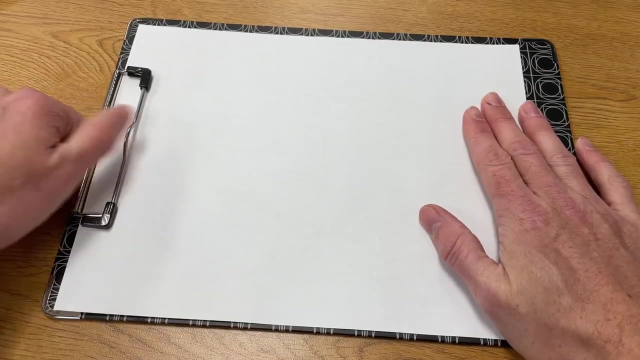 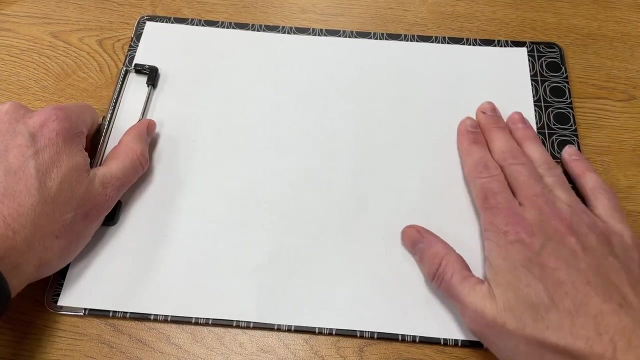 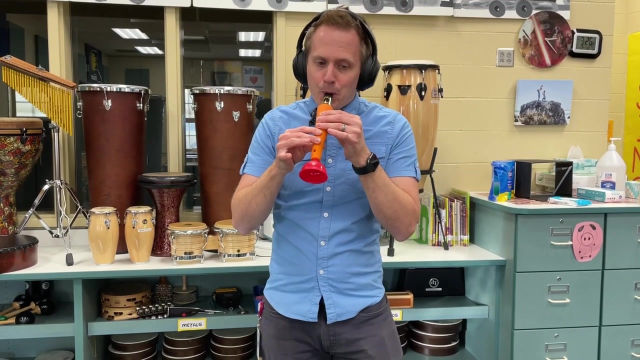 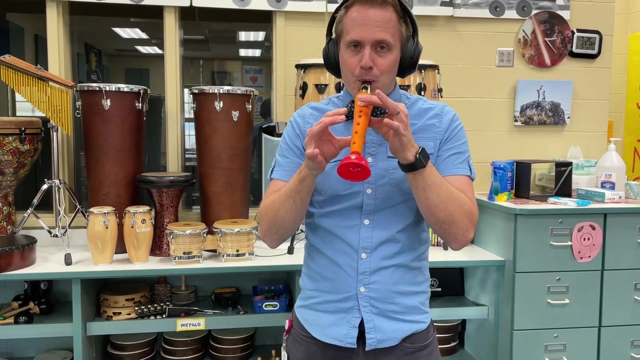 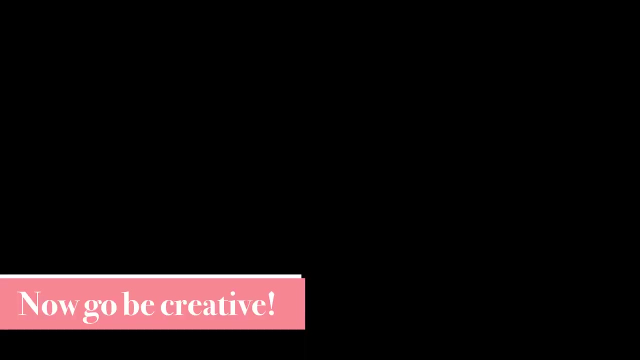 button and subscribe to my channel. I'll see you in the next video. Take care and have a great day. Take care and have a great day, Thank you. Thank you, Take care and have a great day, Thank you.